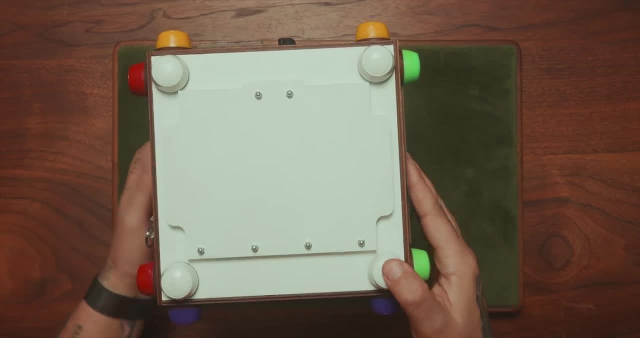 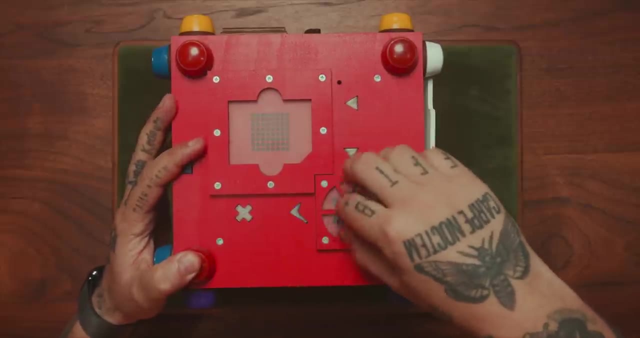 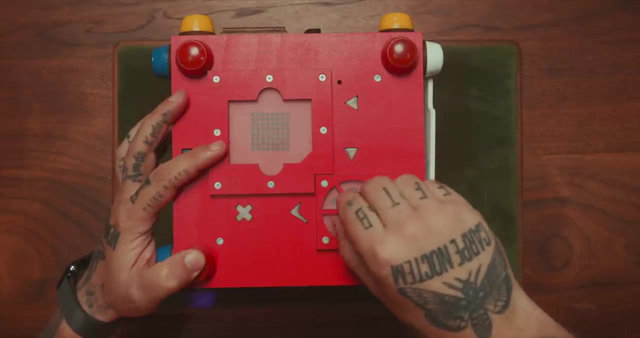 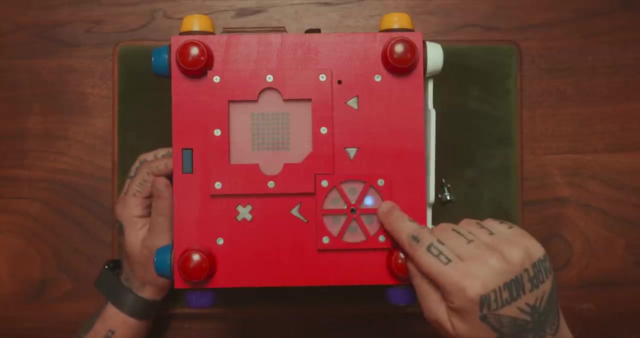 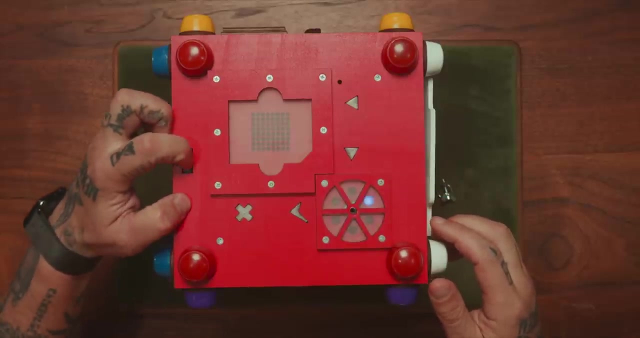 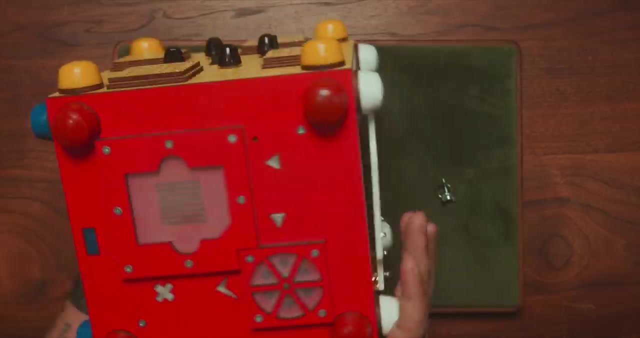 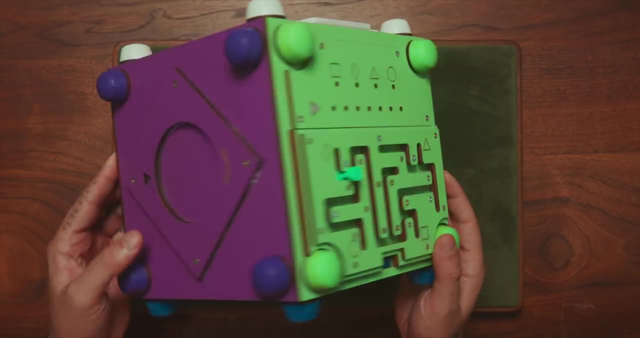 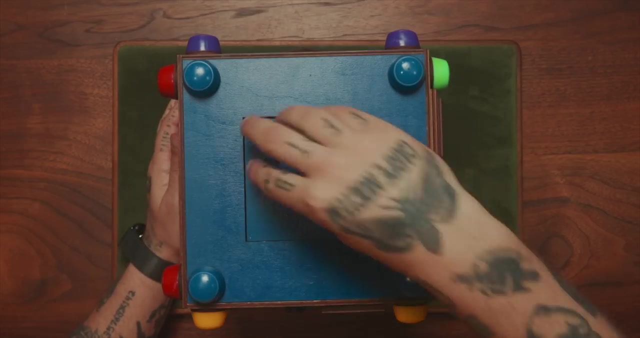 white side, The final panel that will pop open after this is completed. So let's get it started. There might be some music here. Oh, what was that? Oh God, Okay, We have a little light flashing here. Okay, Okay, Some pretty sweet music here. Does this go here? That looks like it might be a fit. 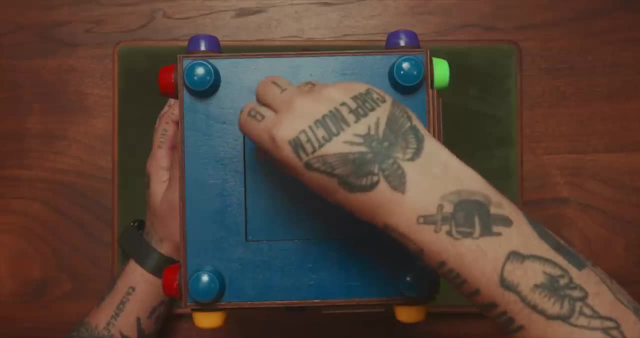 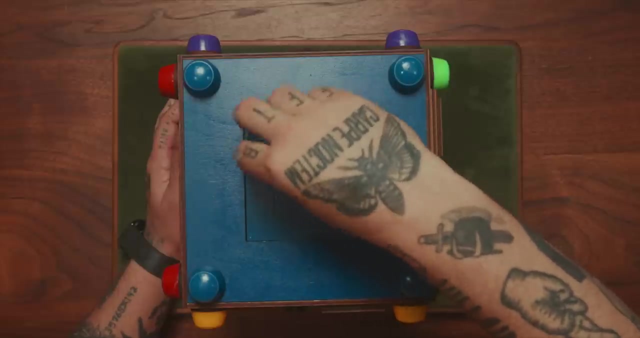 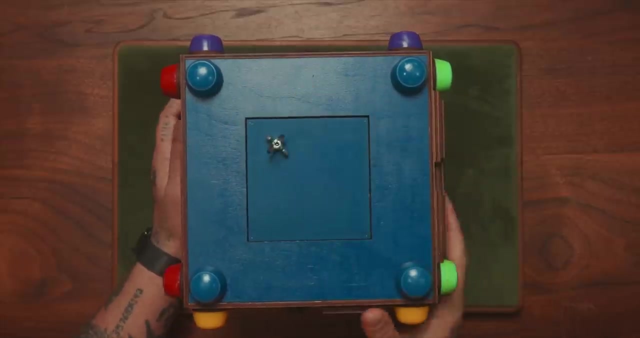 Hey, if you're ever wondering what can I do to help these channels out of this content I really like, Well, just like the video. Like the video, drop a comment, subscribe. That's the type of stuff Really goes a long way. All right, Well, that doesn't really do anything, So 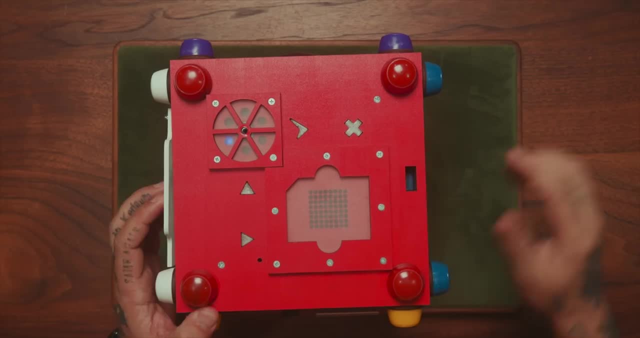 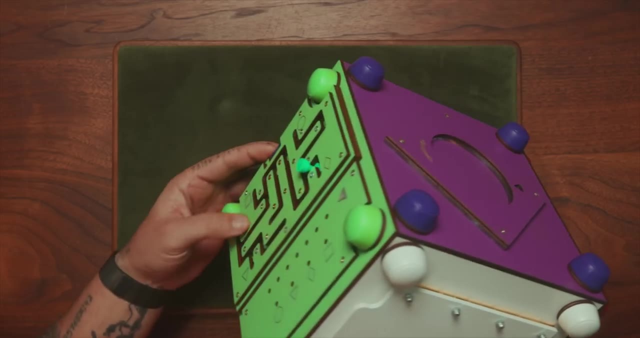 we'll leave that there for now. Maybe that'll do something after. Okay, Well, I pushed that in. I'm not sure I'm supposed to do that, but there you go. Oh wait, It comes out the other side, Oh. 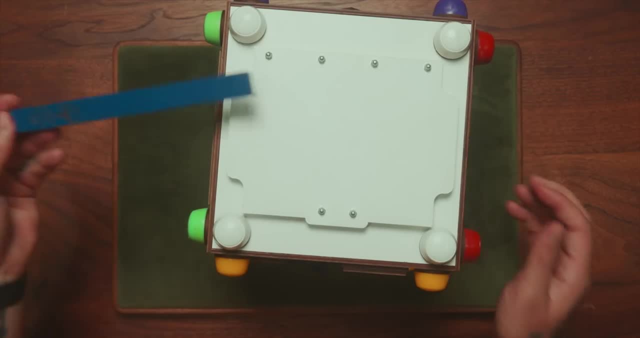 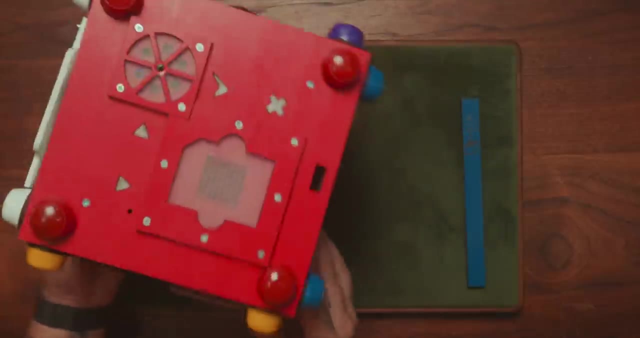 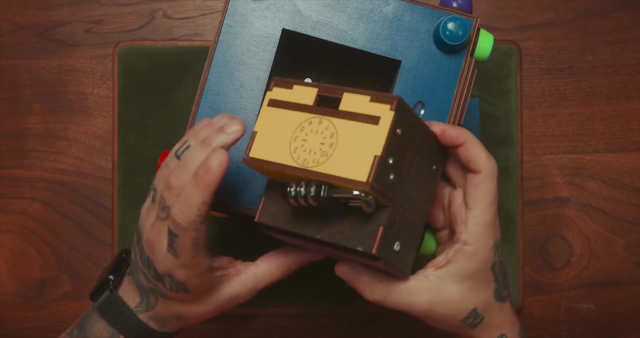 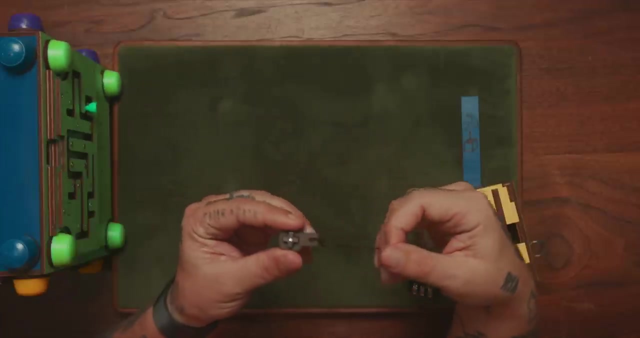 here we go. Okay, It's showing me I've got to use my muscles to pull out, to pull this out. Oh cool Dude, that's so sick. They never ask you to force anything. So happy, they asked me to force something. All right, So for now we've got these. 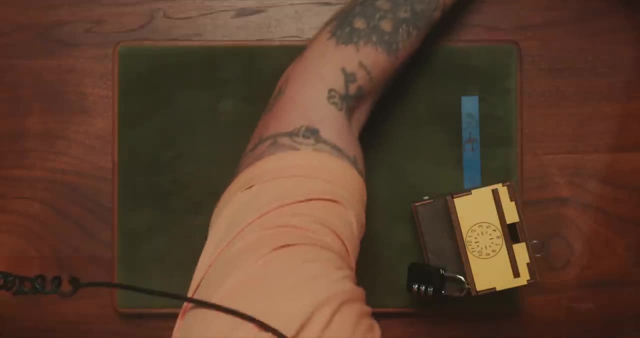 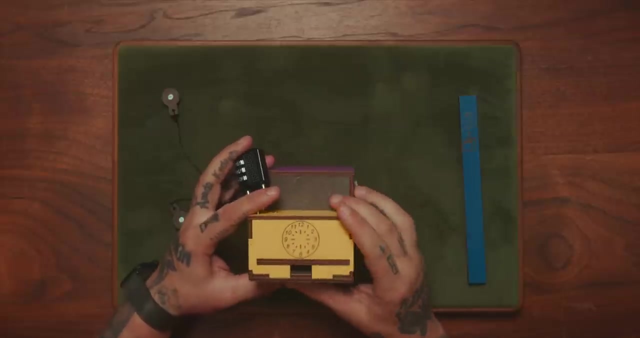 It's so loud, this thing. Let me just put this aside for now. We've got these, Okay, And we've got this. This looks like a face of a clock here. We've got a three-digit combination, Some type of button. Oh, does this go here? 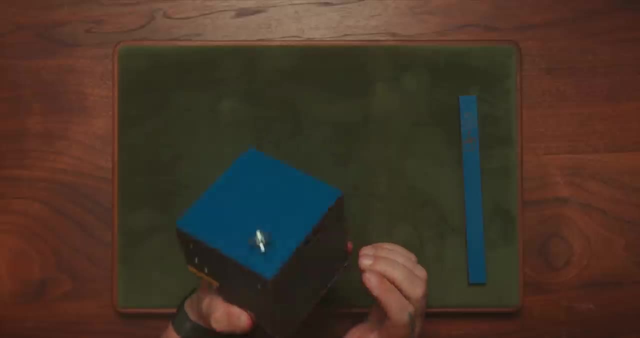 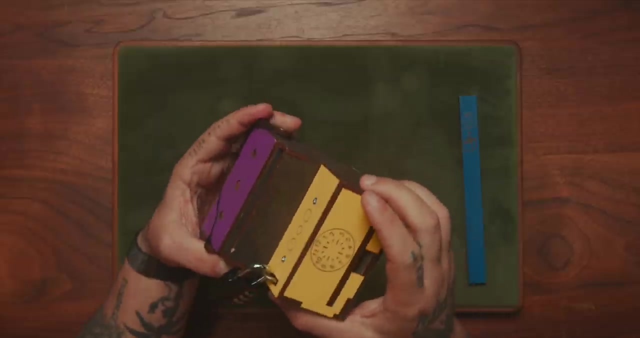 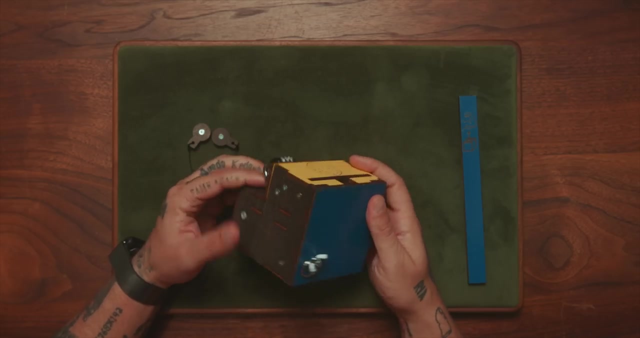 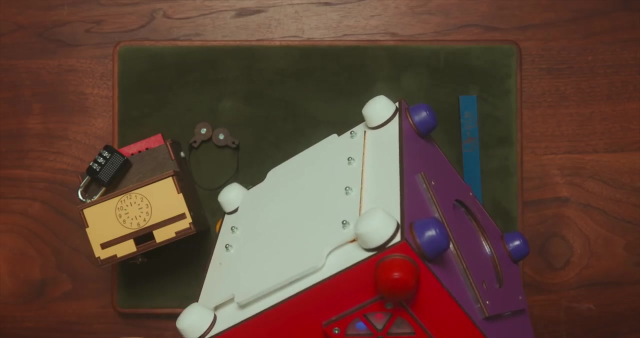 Yeah, There's something on the inside here, Man, this thing is just full of surprises. I'm guessing this is the next step. Okay, Big circle, small circle, big circle. Is that some type of clue? Big circle, Oh, now this red one is flashing. Wait, Oh, so blue meant go on the. 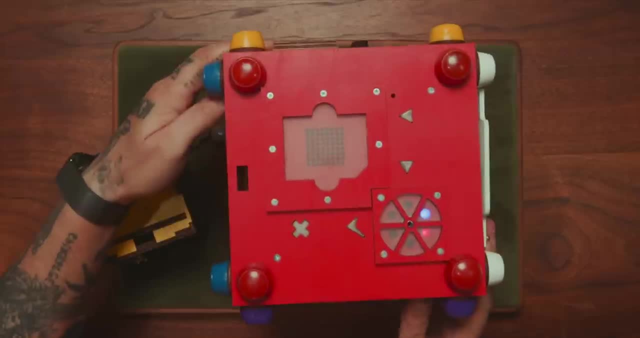 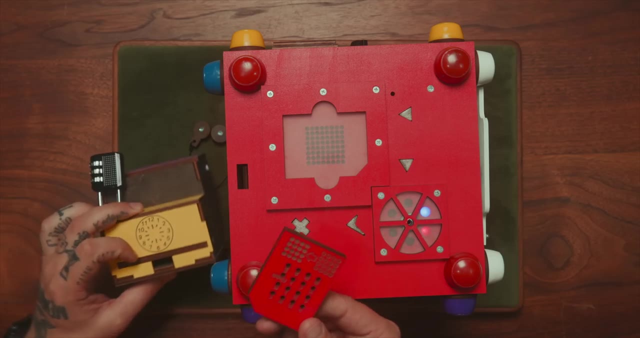 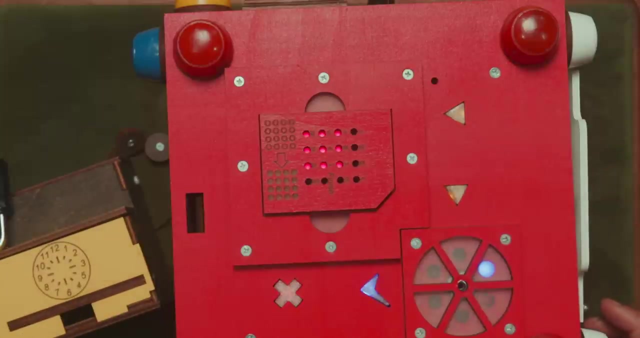 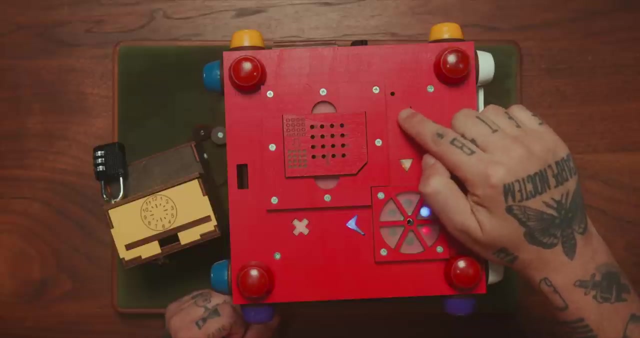 blue side, Red is now on the red side, So now I guess we gotta solve whatever's here, right? Does that make sense? Oh, ha ha ha. All right that one's flashing. So that starts it over. 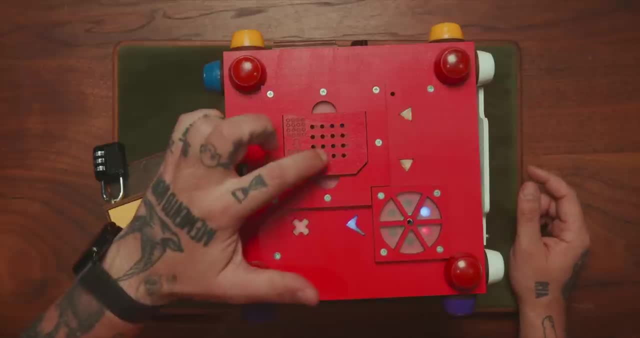 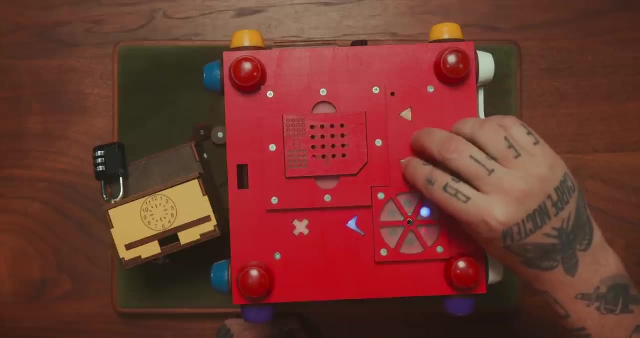 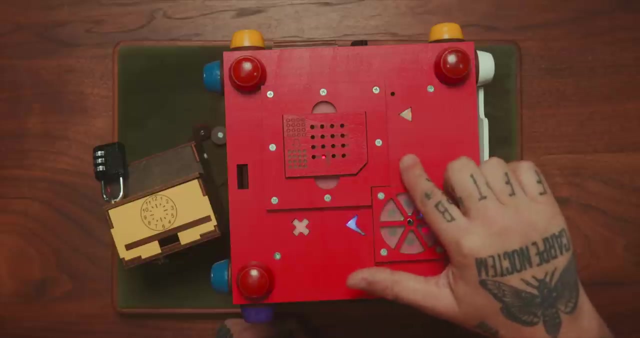 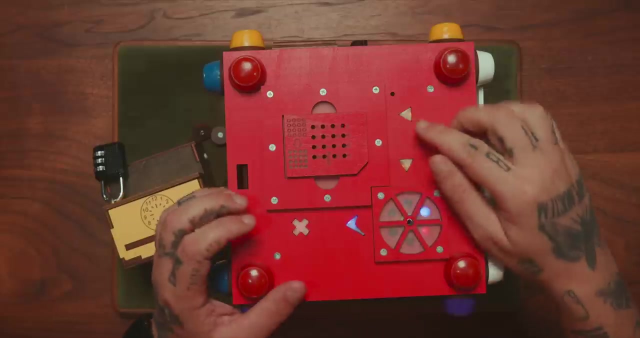 So it goes here. can I just keep going? Okay, there's the finish, Does that not work? Wait what? Oh, so I have to follow the directions. I see. okay, this is cool If I go here. 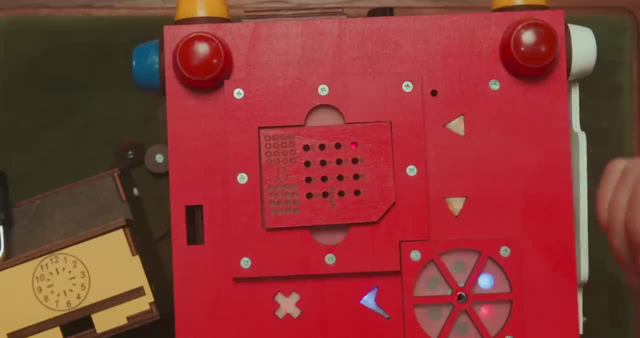 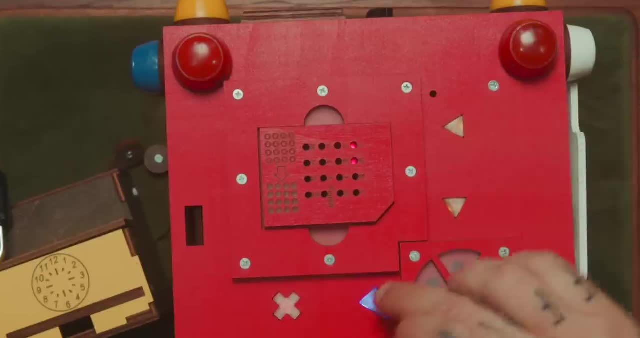 How bizarre. Okay, let's try again. So hit here Down one, hit Maybe one. two hit Up one Hit Over. hit Down one Down down, hit Two over is over here. Up two is there. 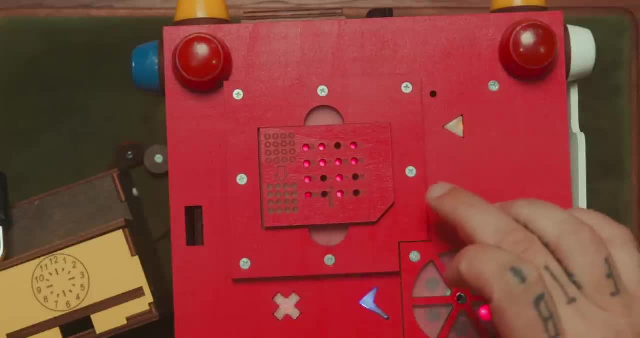 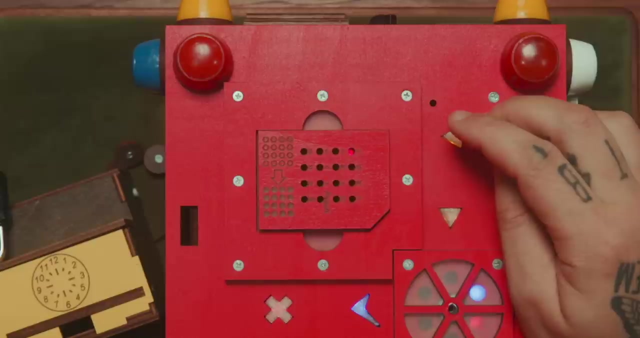 Down, two Over three. One, two, three, That's the next one. So it's there Up, one which is here Over two which is here. Did I miss one? Oh, is it because? oh, we start on that one? 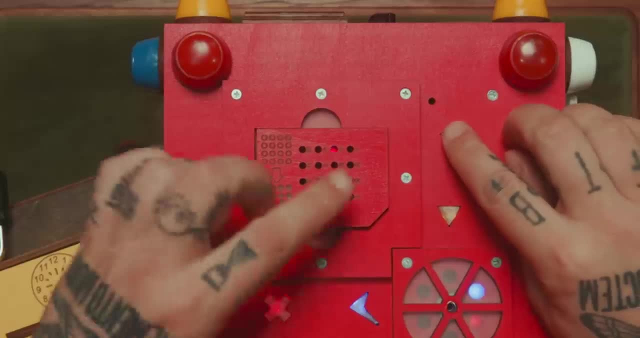 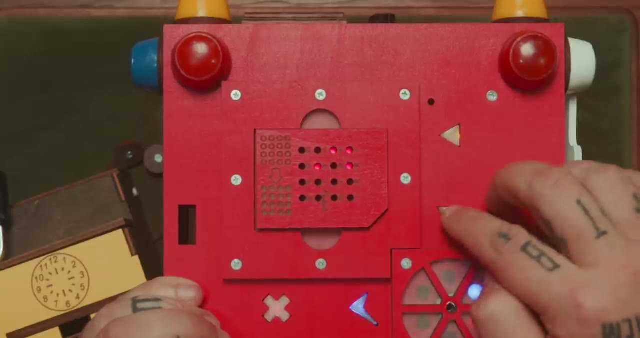 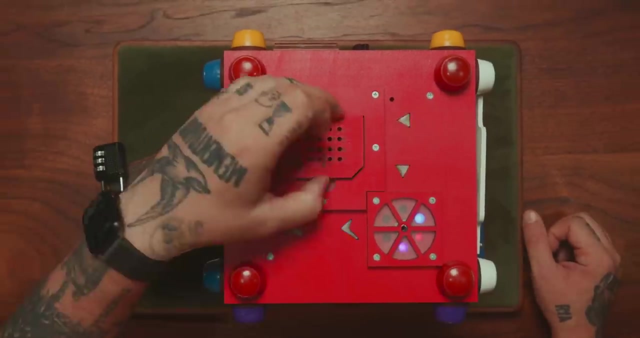 That's what it is. So we start here now we got it All right, and now we gotta go over one. So one, two, three Now. okay, now this is gonna work. Oh, yes, Yes, What now? 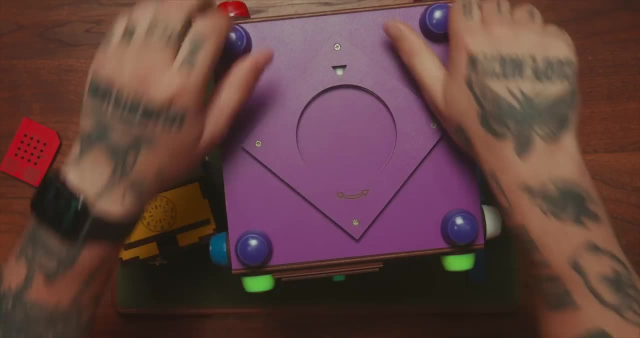 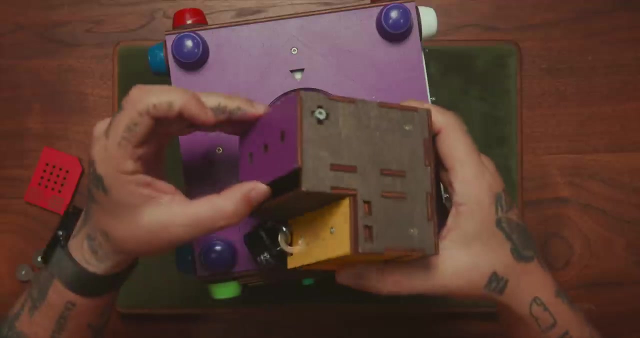 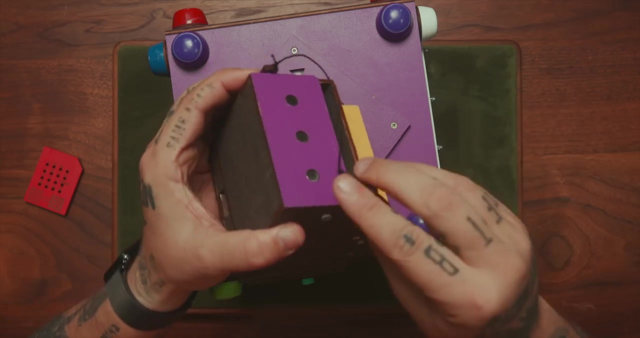 Oh, purple Here. Purple, purple, purple. Why is this saying turn? Maybe I have to open this up first, So maybe I use these. Hold on a second. this goes here Now. this goes here, And maybe now this open. 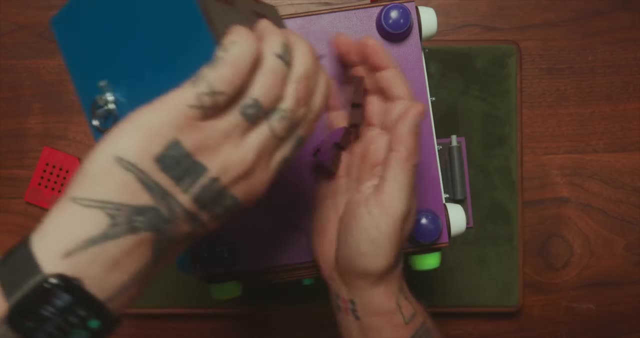 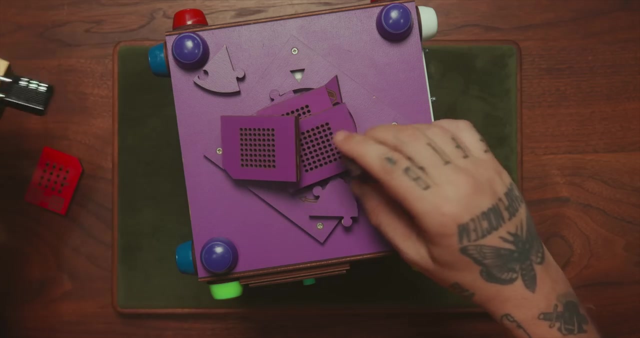 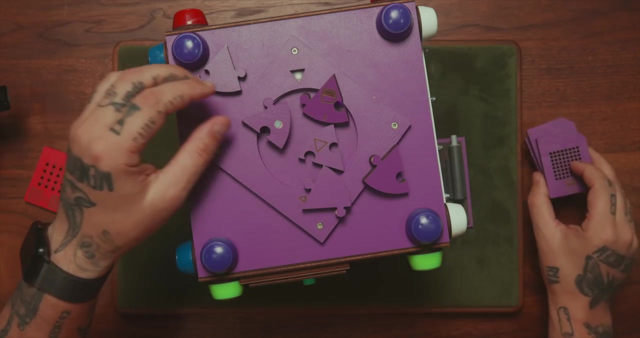 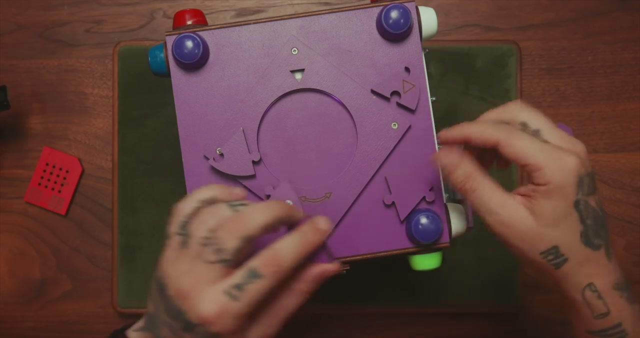 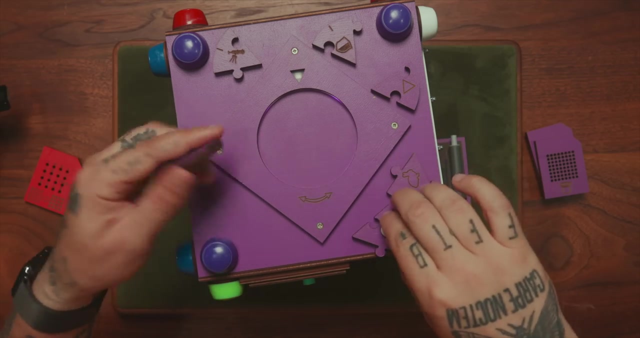 Yes, Oh cool, oh my gosh, okay. so I've got these things as well. we've got a top hat, a sword and a star, and then we've got these, and this one has a thing on it. okay, we've got a triangle here, a bunny, a telescope, a shield. this one just has like a knob on it and this one has nothing. 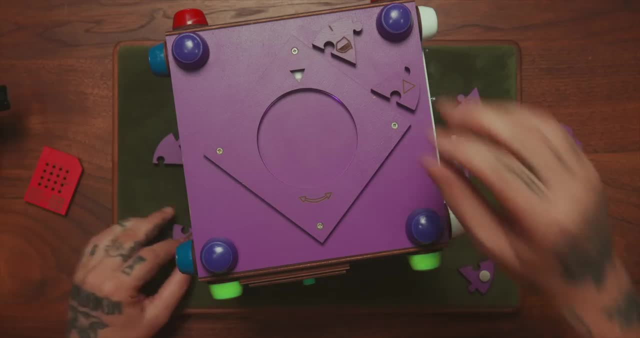 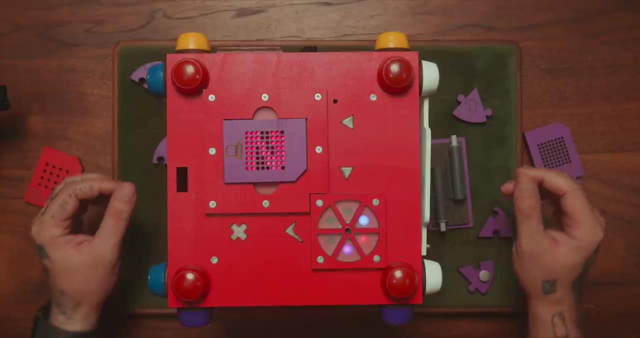 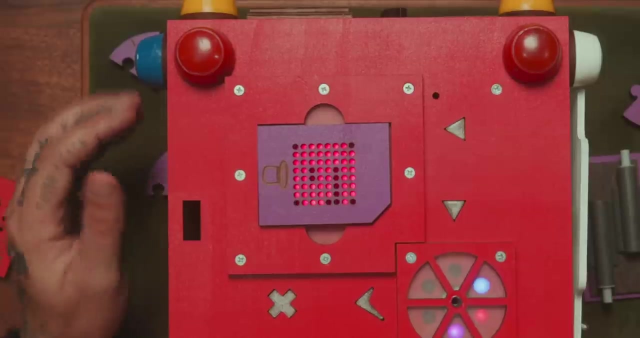 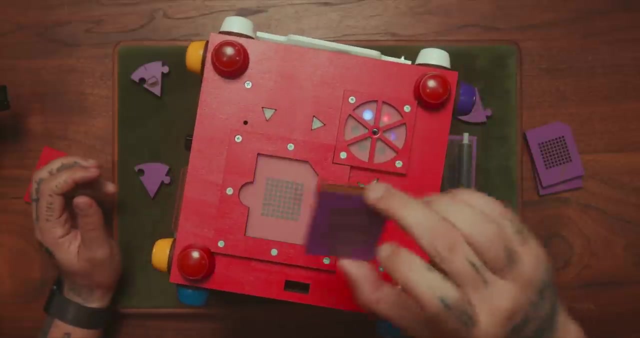 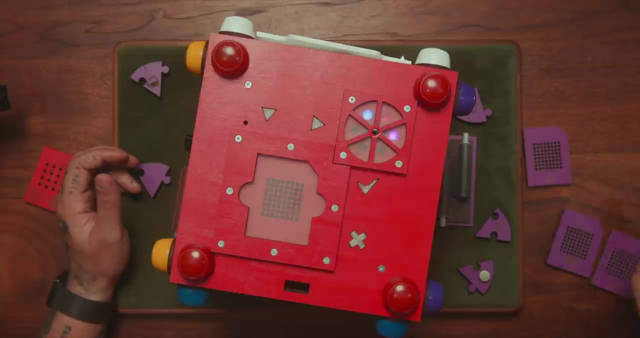 okay. so I'm thinking, first of all, let's try, and, because this does have the same shape as that other thing. so this is a top hat n? n. what is that n? what? z? 26, 26, 26, this is 26, it's 26, okay. 35 or 53, 35, 26, 35, 14. 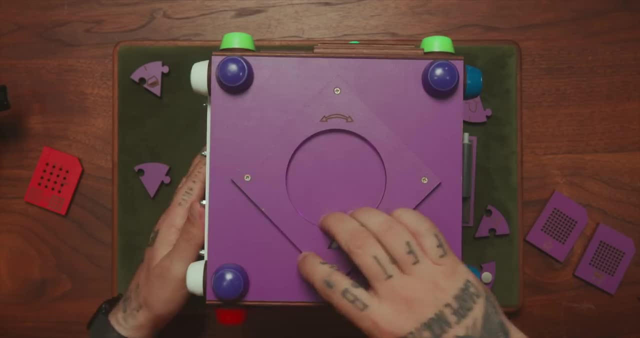 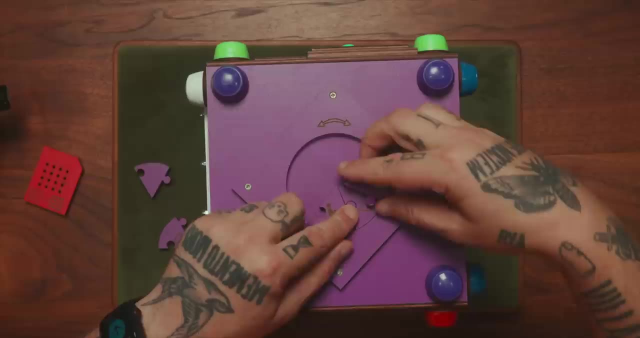 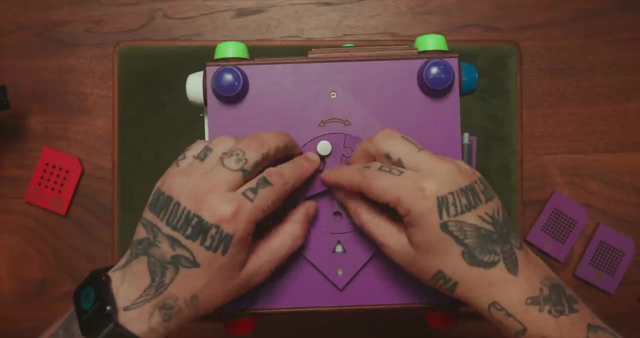 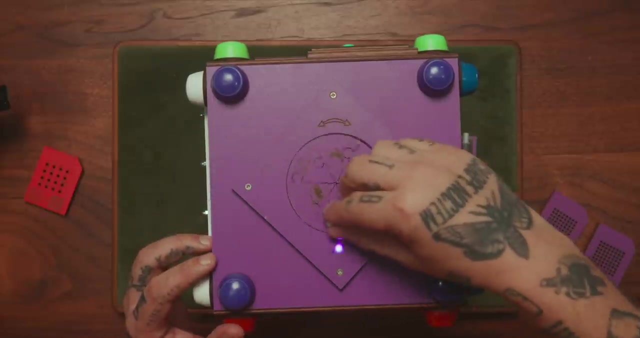 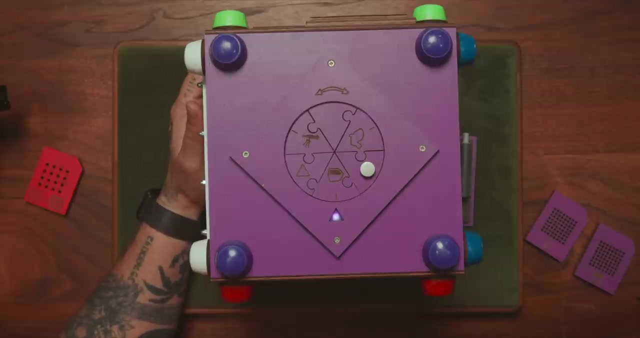 okie dokie. so I gotta figure that out now. well, let's try making a circle actually easier than expected. so this goes here and no, this one, yes, now this one, uh, and this one that light lights up. oh, the sword goes with the shield, the star goes with the 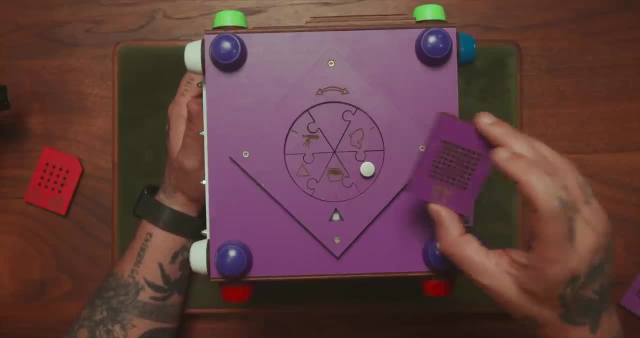 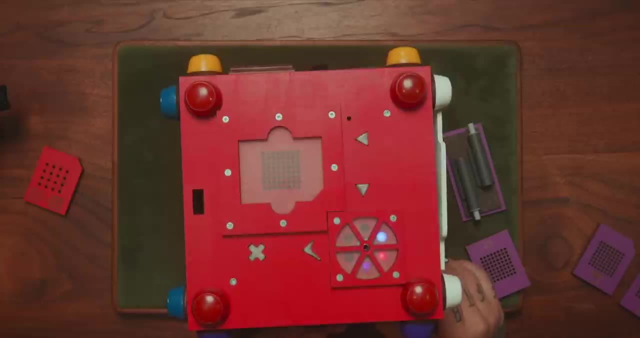 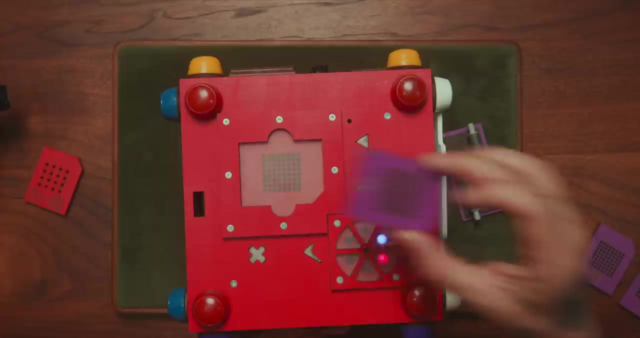 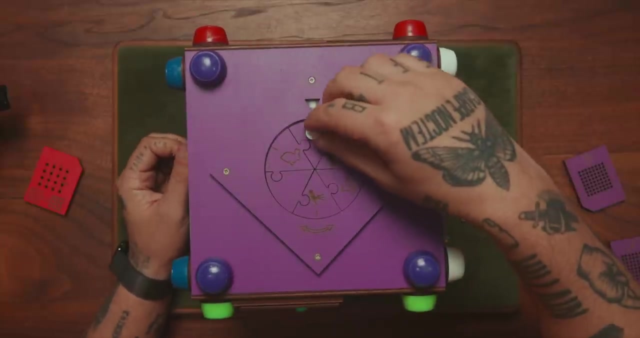 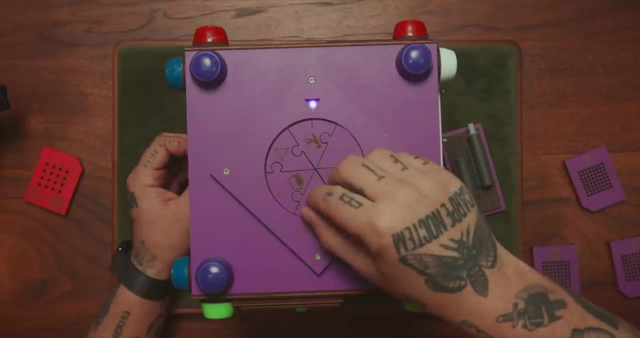 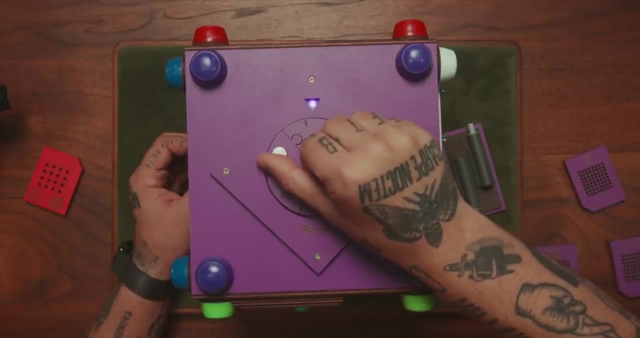 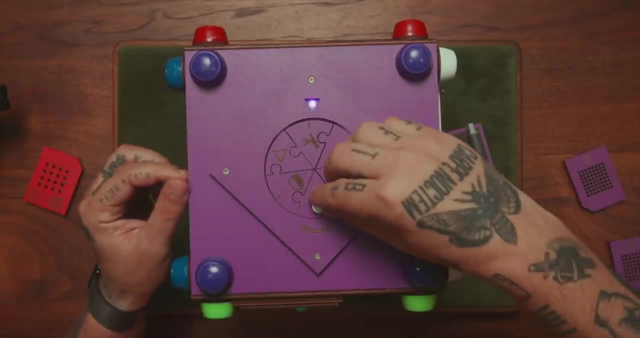 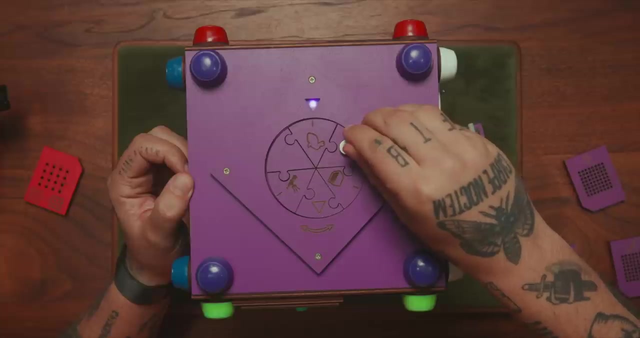 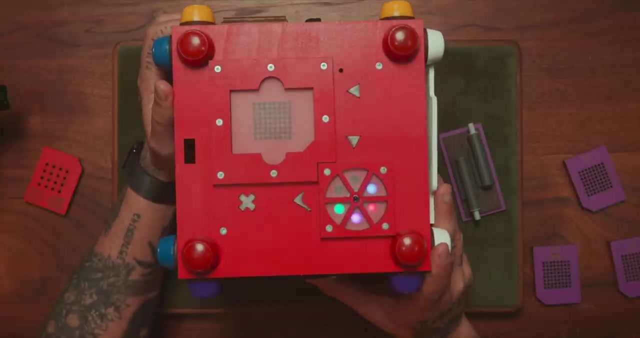 telescope and the hat goes with the bunny. okay, this is a starting point. it's a combination, wait, wait, oh, one and four, two and six, ah, so it goes. star hat, sword, star star. Completed, Is that not it? yes, let's go. I think the sound bugged out, not getting any sounds. 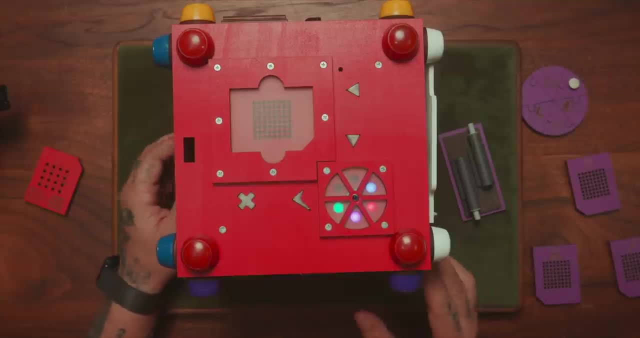 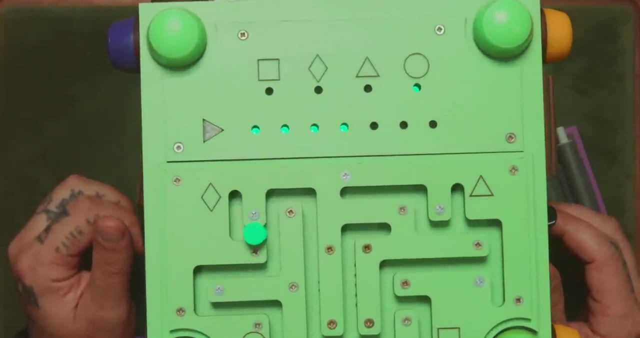 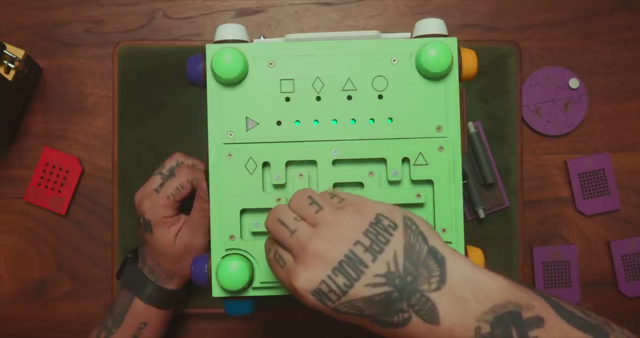 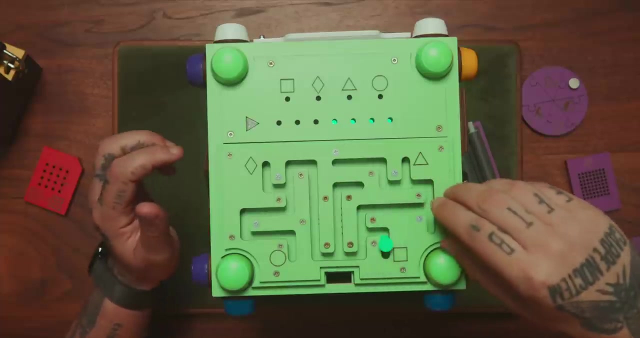 which is nice. I didn't really enjoy that music. anyways, we're on green now I So diamond circle square, circle triangle, circle triangle, Diamond circle square. diamond circle square. diamond circle square. I have to do it in one sequence. 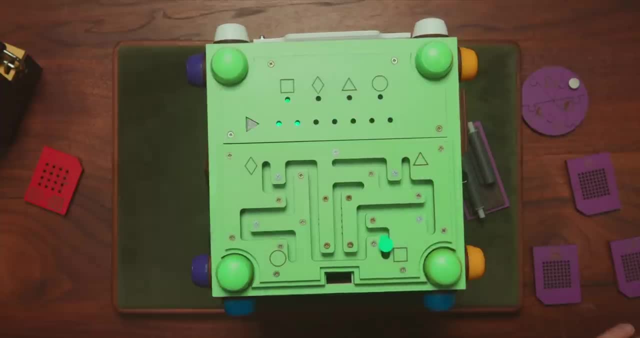 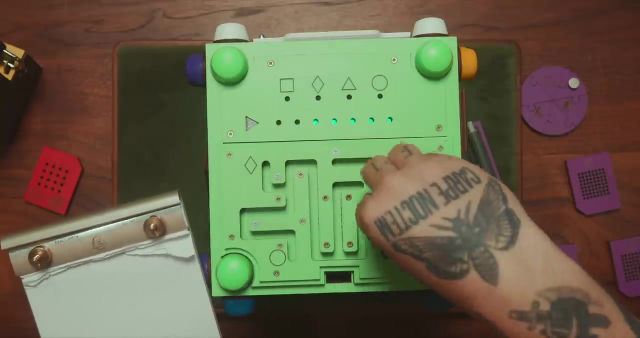 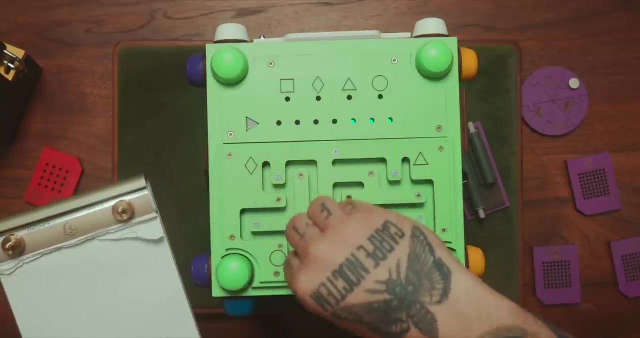 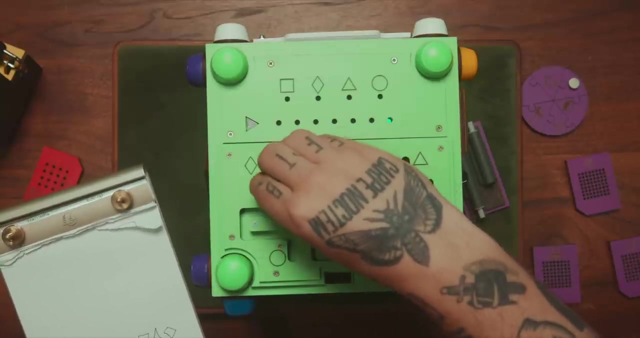 I can write this down My trusty notepad: Let's go Circle square triangle, circle square triangle, diamond, circle, square triangle, circle, square triangle and diamond. for the finish, I have to do it in one sequence. 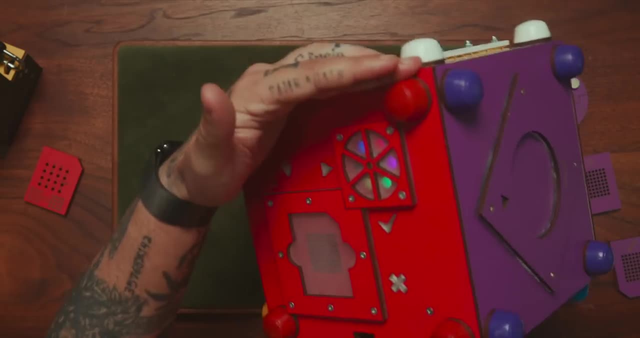 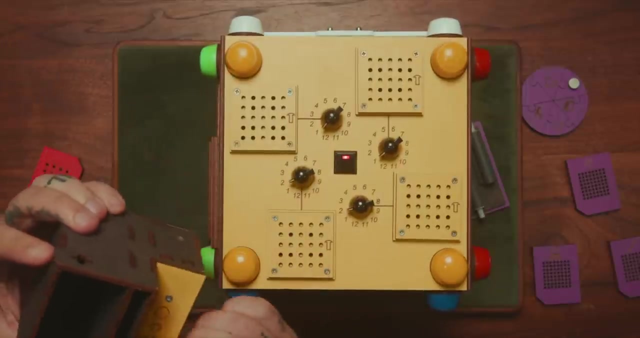 Yeah, Oh, now it's flashing yellow, So we go to yellow, which is here. This one looks complicated. We got this as well. We've got like a clock here which matches the clocks here, And then we've got three individual circles. 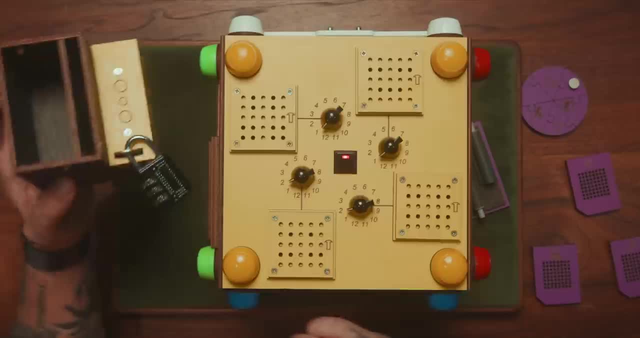 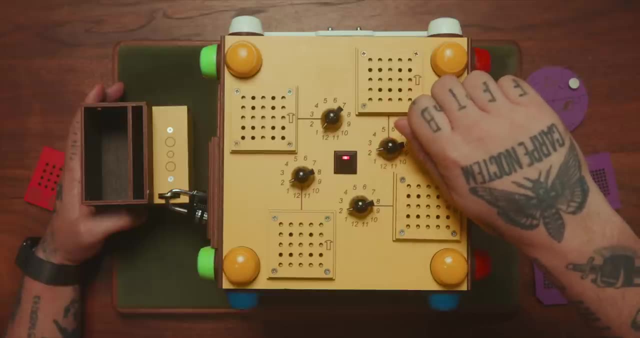 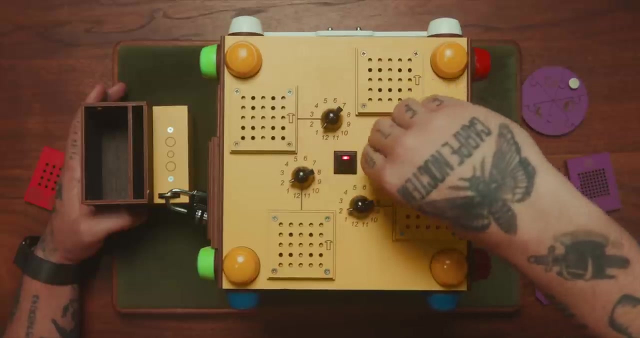 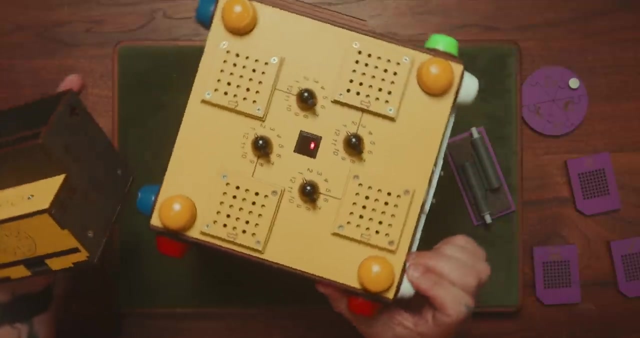 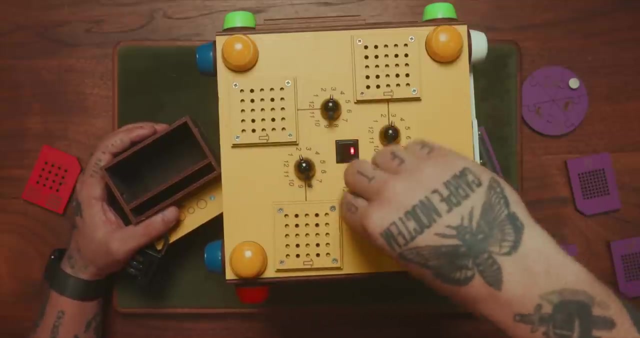 So I don't know what they mean. We've got arrows on these things And we've got a three-digit combination, So Okay, So they're all starting at one o'clock right about there. Now you can notice there are little holes. 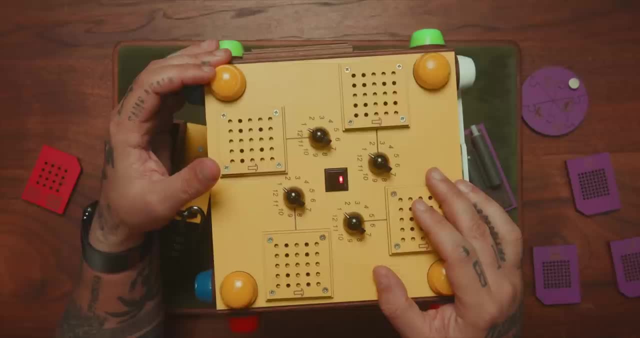 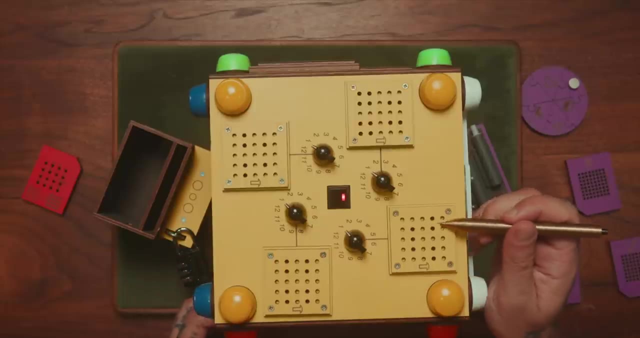 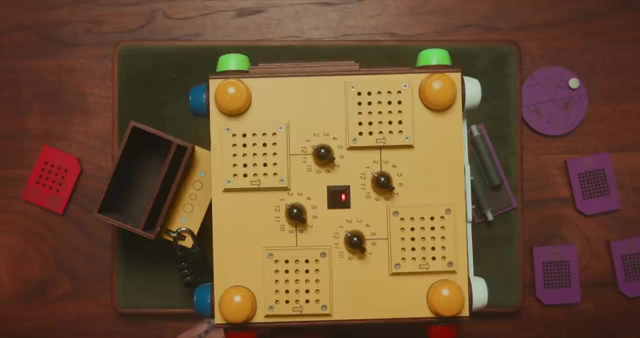 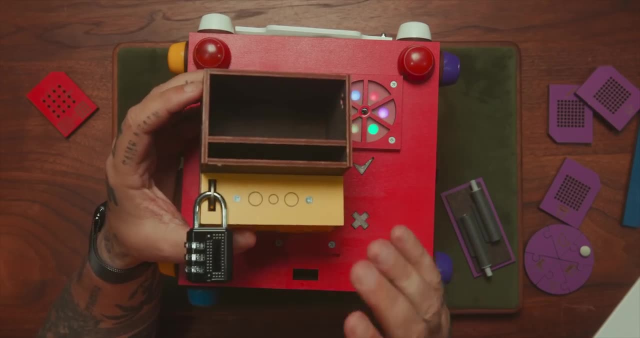 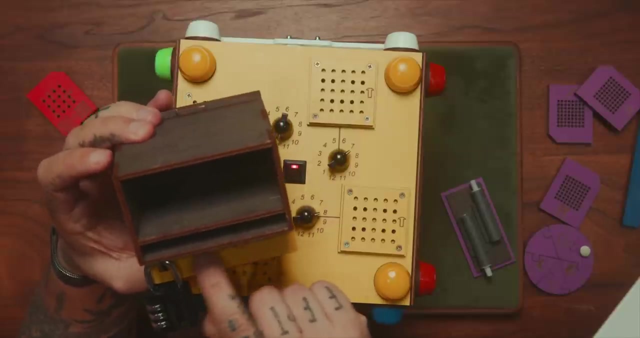 Now I'm wondering if in the negative space there might be some type of number, but it doesn't seem like it. Pretty sure, whatever it is that I need to complete, the yellow side would be in here, And I'm pretty sure that is the combination. 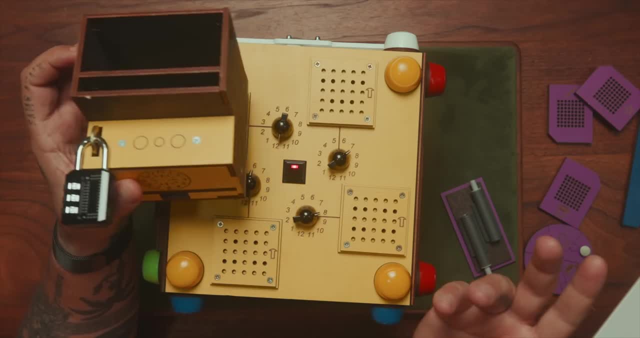 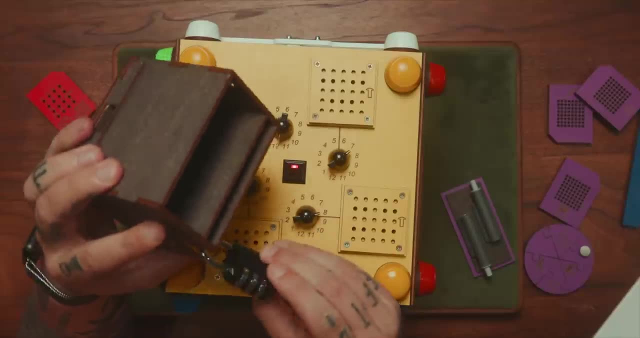 So two numbers that are the same, One number that isn't, But other than that I have no way of knowing. We'll just do, we'll go 1, 0, 1.. 2, 0, 2.. 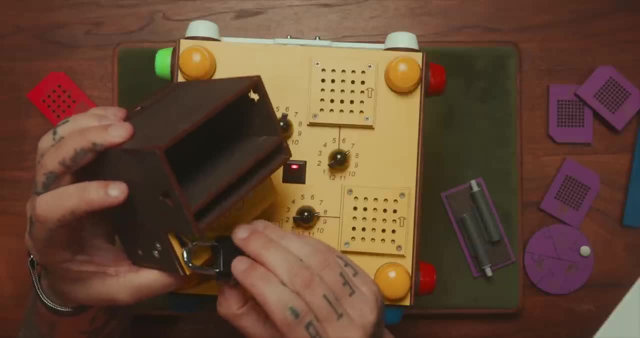 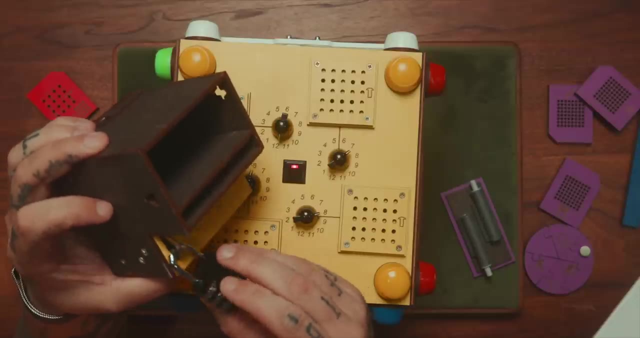 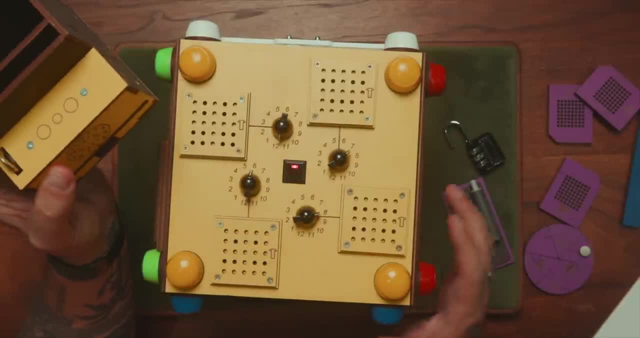 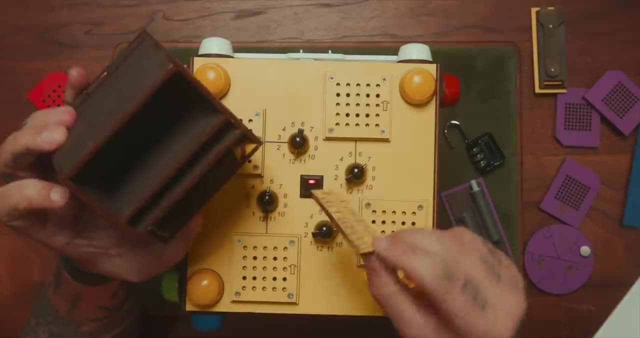 5, 4, 5.. 5, 4, 5.. Oh, we got it, Okay. Well, I hope that wasn't the solution, because I'm obviously missing something really simple somewhere, But I didn't seem to find it. 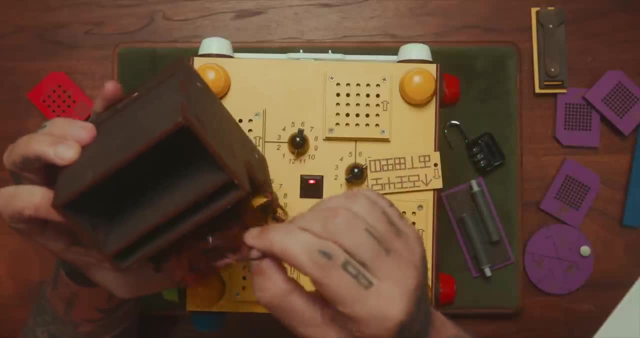 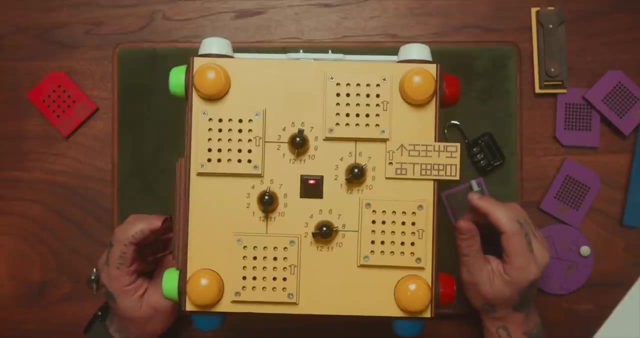 But we brute forced our way through, which is totally acceptable in my book. What is all this? Oh my God. All right, Okay, Arrows up. Oh, they're numbers. You see the shapes I drew out before. That would be like two numbers. 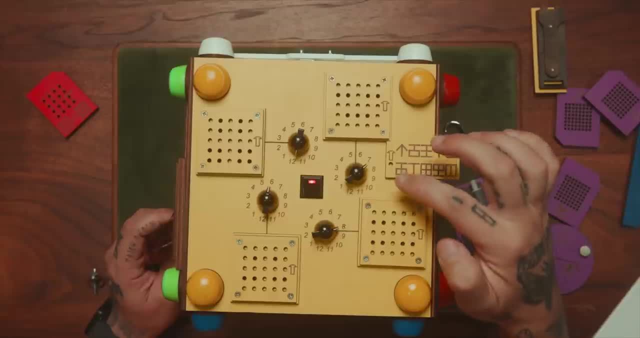 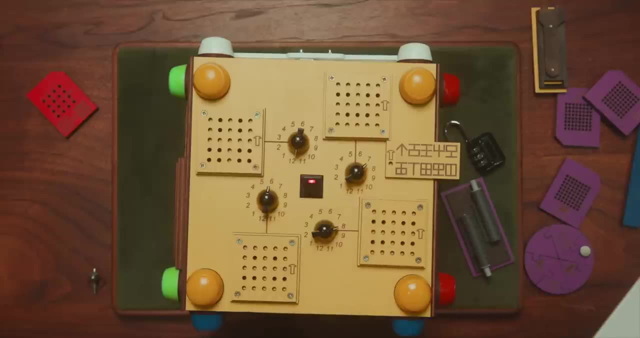 That would be like 2,, 3,, 4,, 5,, 6,, 7,, 8,, 9, 0.. Oh, maybe I wasn't supposed to see that some of them were depressed a little bit, Could that be? 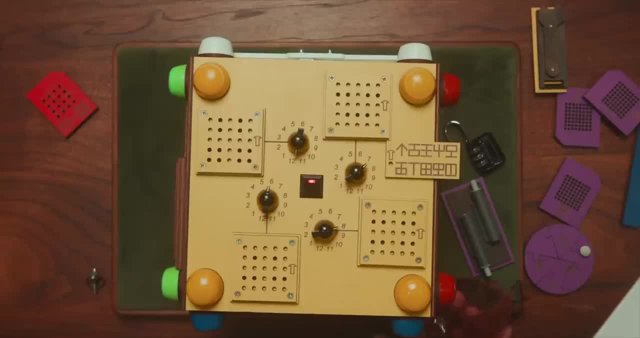 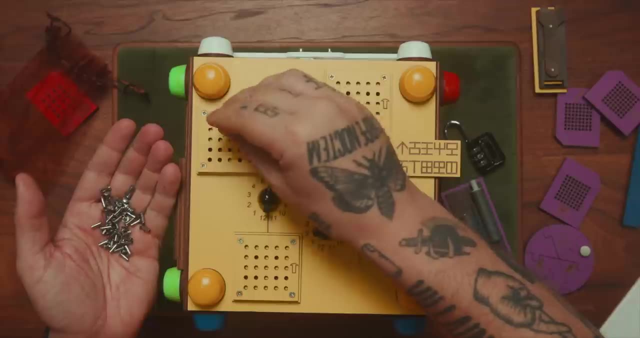 I don't know, Maybe no, That's impossible. And then we have pins. Let's take these pins out. Oh my God, So many pins, All right Numbers. we need to get All right Here This one, And if I put it in here, would it be up? 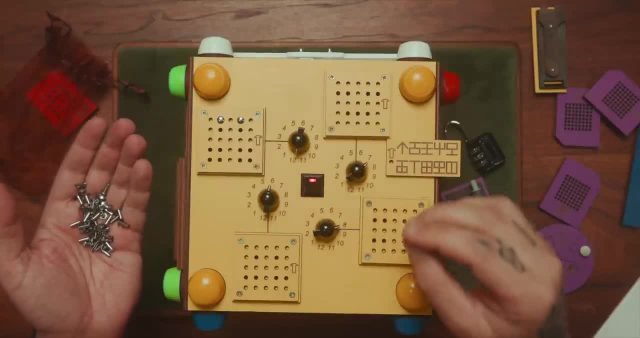 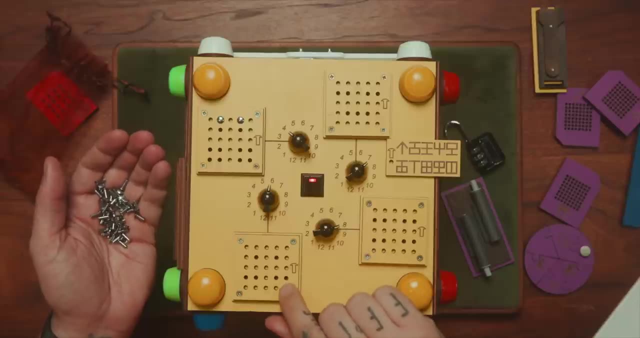 Yeah, it would be up. Okay, So here Is this meant to help us figure out the numbers, Because I don't even think I need this Right now. This one's four, You can see it: four. This one would be five. 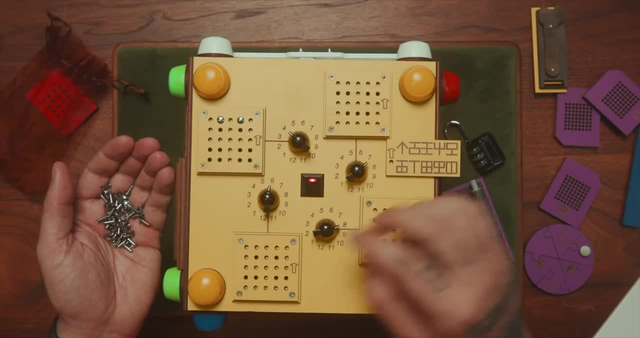 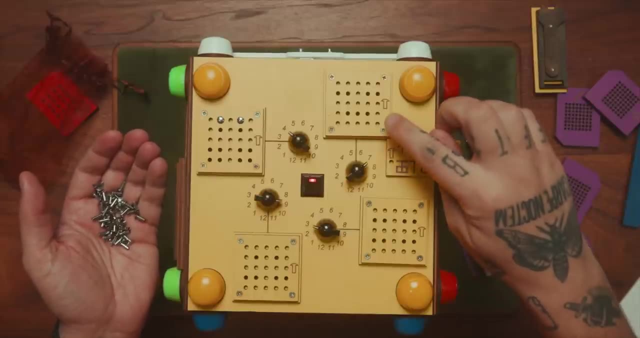 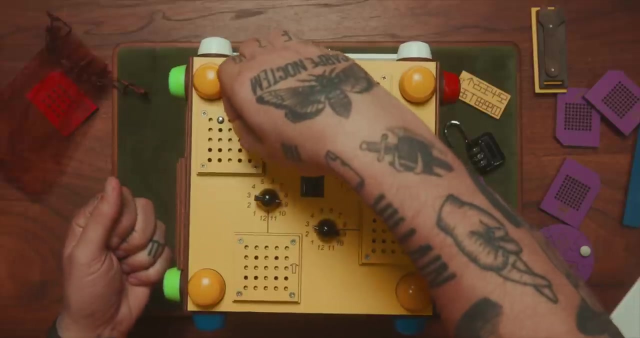 Right, Like this. There's a line in the middle and this one would be nine, This one would be three And then this one would be two. Did I do it? I did it All. right, We don't need these pins then. 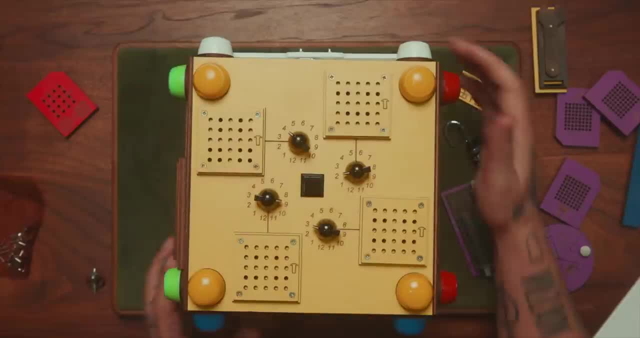 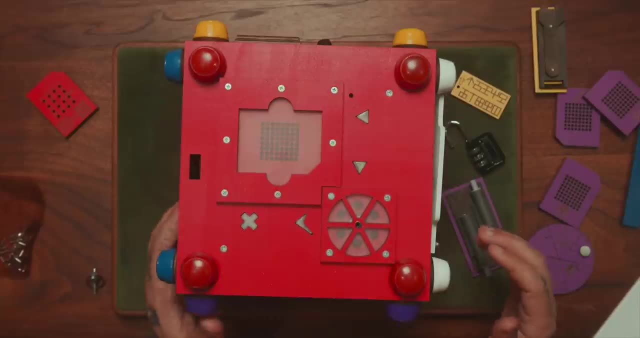 Those are just, I guess, markers to help you see them more clearly, because they are quite faint. All right, It now says red, Oh, Red, Blue, Yellow, Purple, Green, White, Red, Blue, Yellow, Purple. 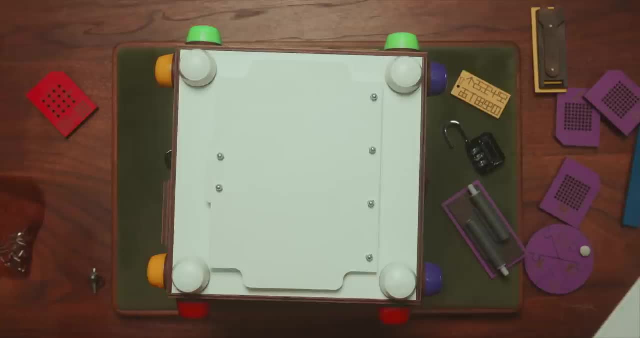 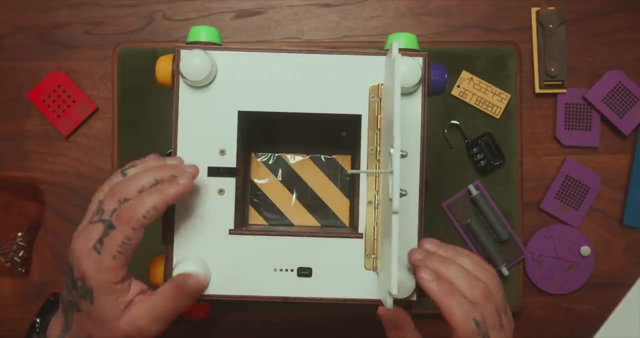 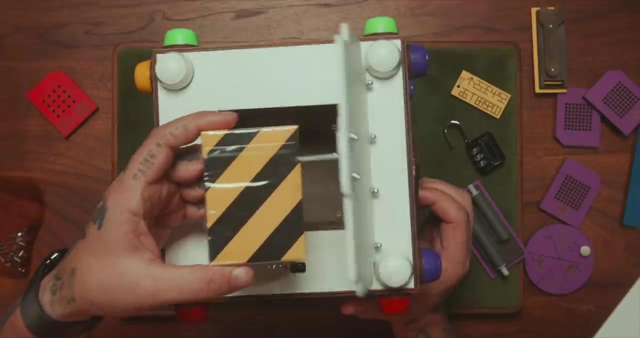 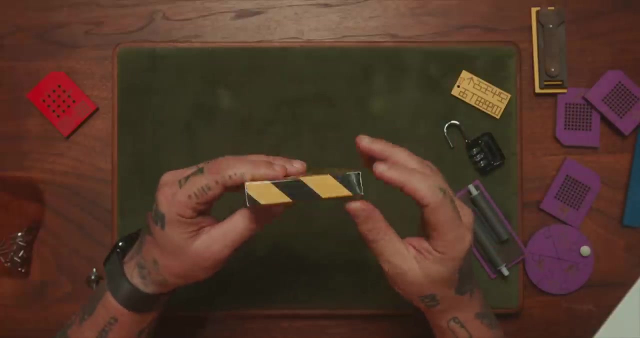 Green White. Oh my God, I got a surprise in here. This is so funny. Antoine put, I guess, Wes' second playing cards in here. These are Wes' deck. You know, I love a good surprise. That was actually quite fun. 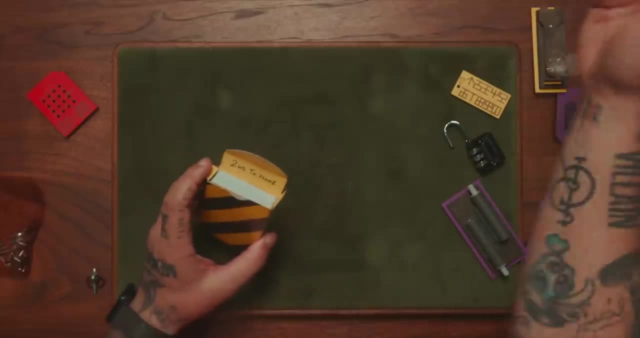 If you want to check these out, these are Wes' playing cards. Second to none. They're available at WesBarkershop. Wes is my best friend and these are his cards, and they look pretty cool. This is the censored deck. 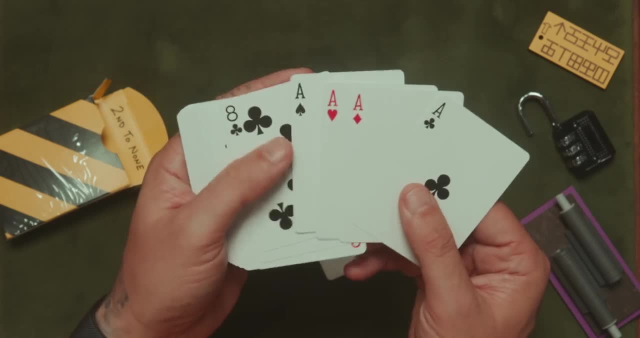 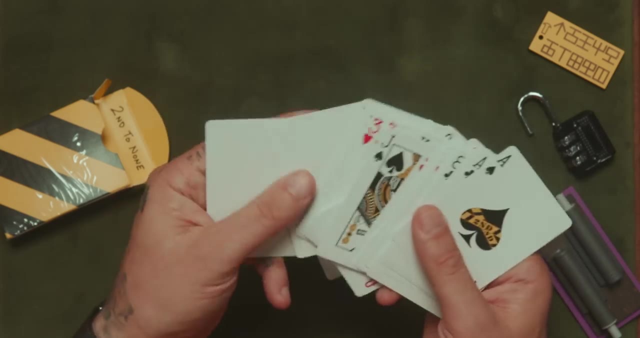 These are the jokers. They come in alphabetical order. by the way, if you're wondering, That is the ace of spades, Really nice cards. And then The core cards. all have censored. Two blank cards for some magic tricks. 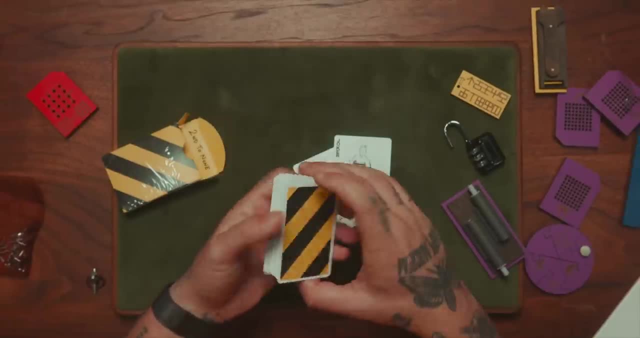 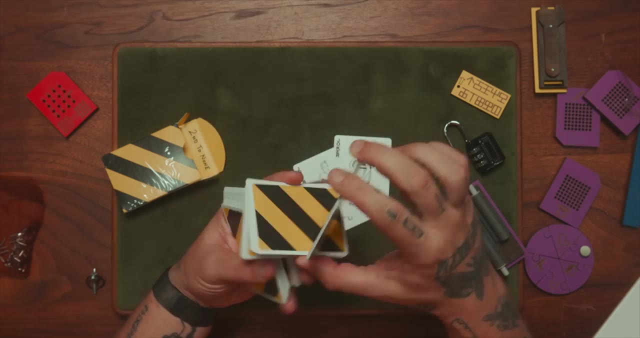 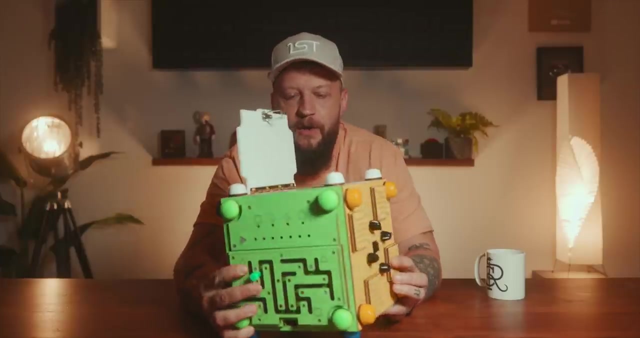 And the back design, which reads little seconds here. They are super, super sick, looking by the way, Whoa Printed by the United States Playing Card Company. so you know the quality's good. Well, hot dang, here we go. 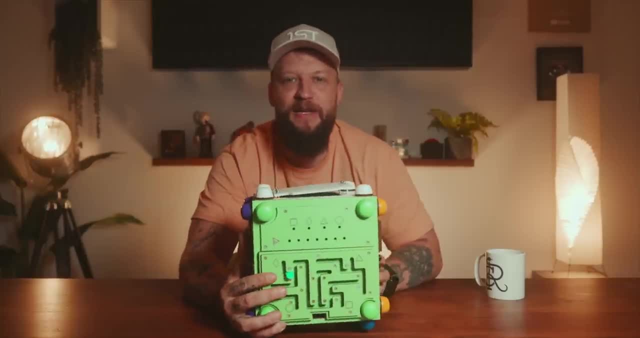 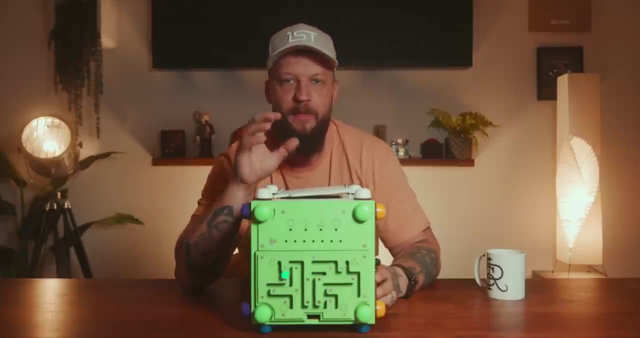 This is the puzzle solved. So inside, Antoine left me a little gift, which I always do appreciate, But that was a lot of fun. I did get stumped at the yellow part a little bit because of the combination. I'm still not sure how to.